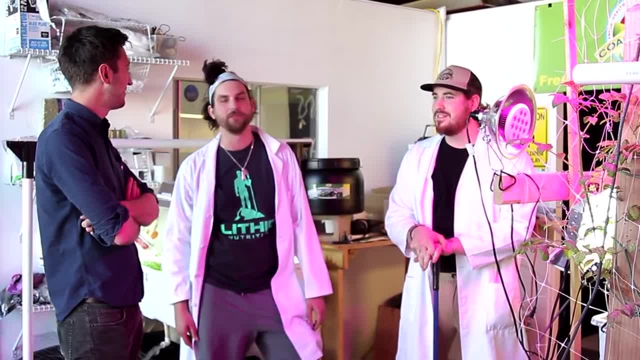 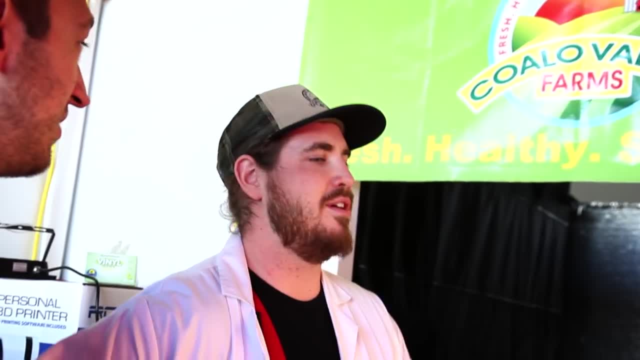 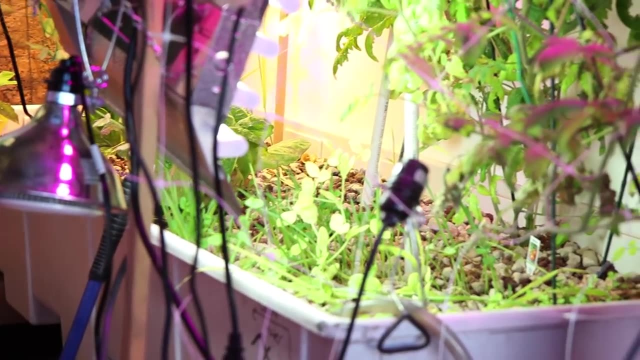 own little niche so far and ours kind of focuses on the green and just kind of the more a different style of farming altogether. These crickets are literally the happiest crickets you'll ever find, Pampered- I would say pampered is the word. The crickets at Koala Valley Farms live on a. 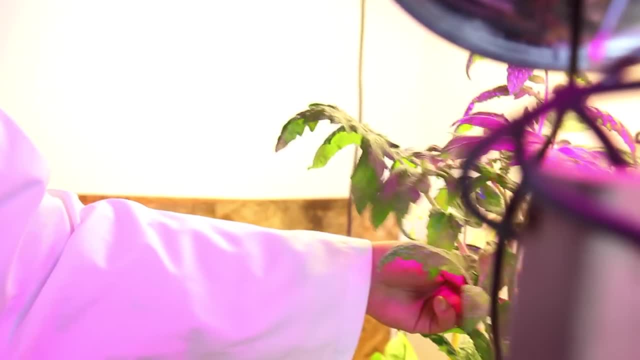 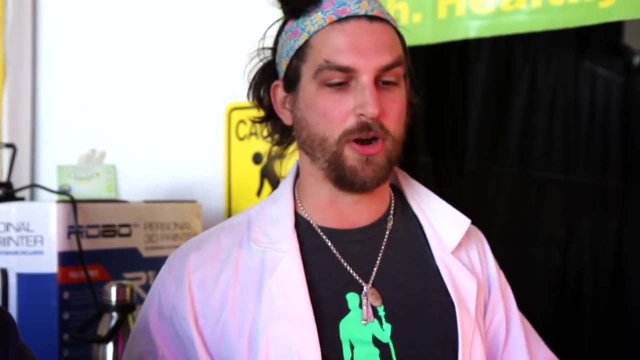 diet of fresh veggies grown for the most part directly on the premises. Our crickets are vegan crickets. Do other cricket farms feed their crickets like meat? All cricket farms abroad and most cricket farms here feed their crickets chicken feet. You're basically eating corn. you're just removing yourself one. 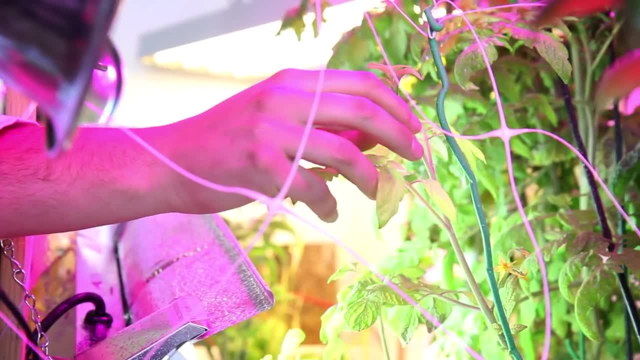 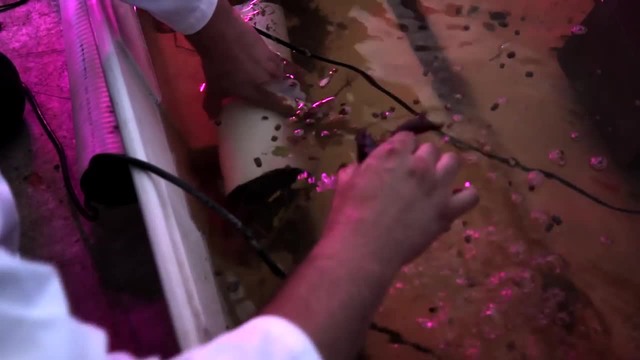 step from it. The vegetation is supported by numerous aquaponics systems, in which the water used to hydrate the plants is enriched by the bodily waste of fish and crawdads. One time I ate a crawdad- that was, I think it was full of eggs, and then 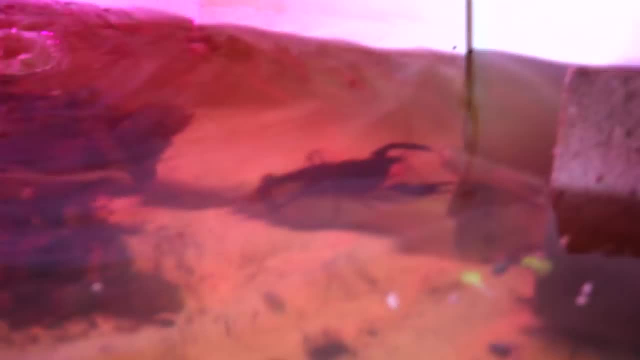 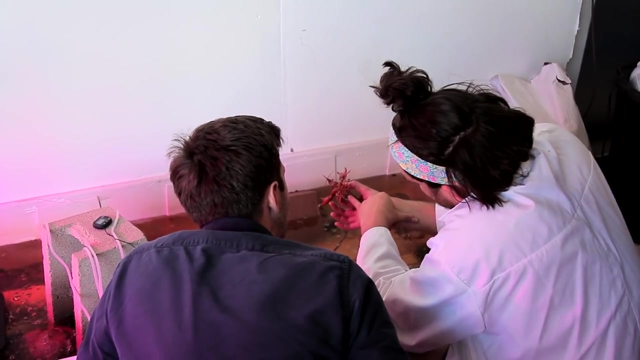 I threw up: Yeah, As you can see, I'm kind of a crawdad expert, but as it turns out, so was Elliot. So this right here is essentially the crawdingus. Wait, that tiny little thing, This yeah, well, this one's pretty big, I mean think. 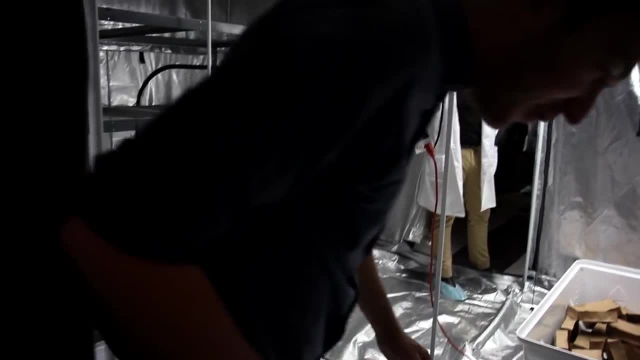 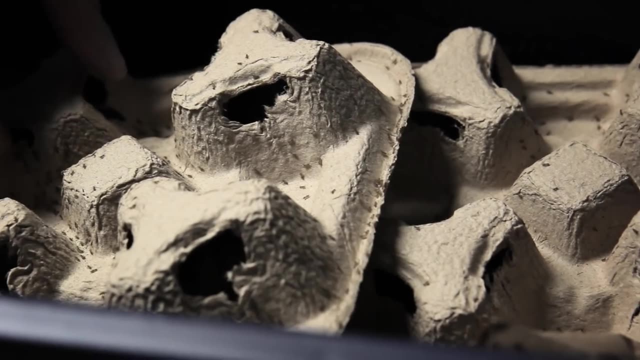 about this. After a few minutes we remember that we're not here to talk about crawdad penises. so Peter and Elliot lead me into their cricket kingdom First up the egg room. Oh, it's so humid in here. Yeah, So how many, I guess I. 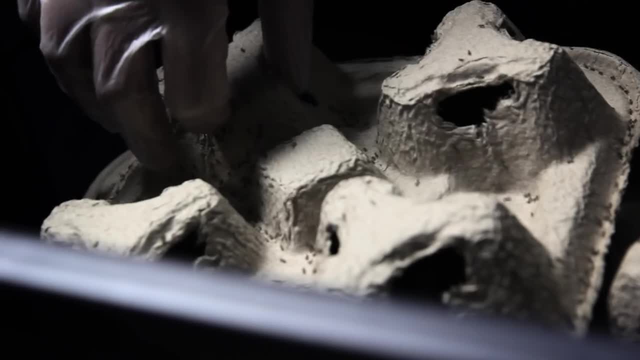 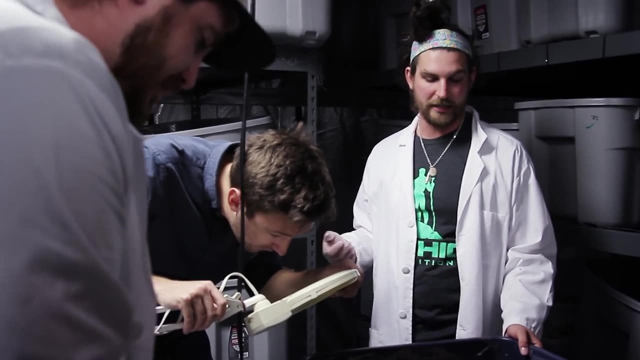 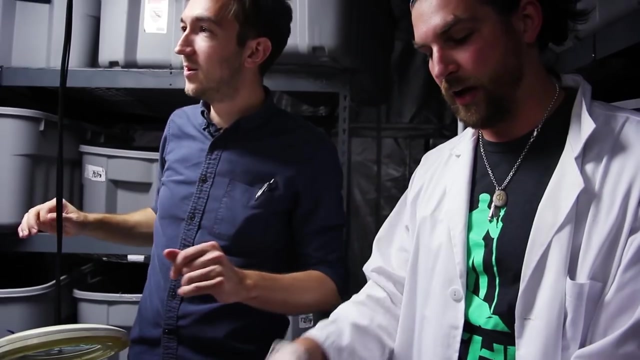 don't even how do crickets? So that's me searching for the words to ask about cricket sex. The males deposit their sperm on the lady's chests and legs. She basically gets erect on top of the soil, humps the ground repeatedly, and with each hump she 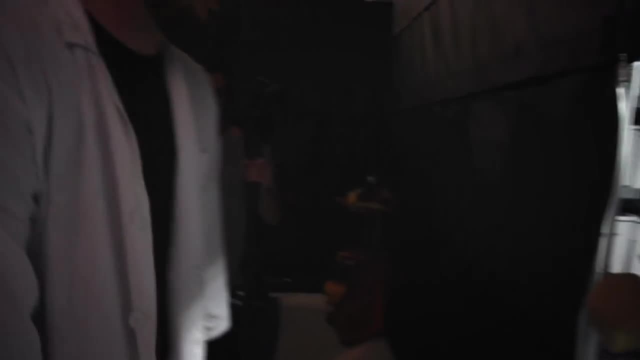 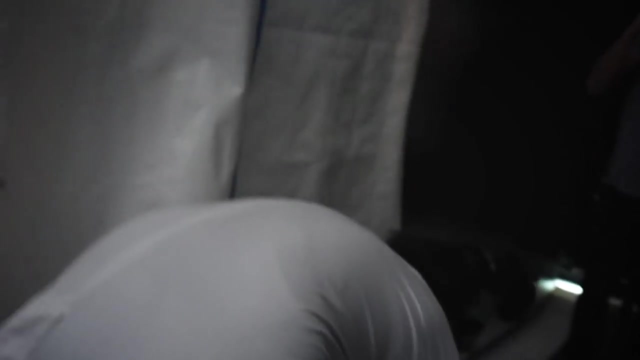 deposits one egg, We'll see some egg laying in the next room. but before then I take the time to ask a tough but necessary question. You're not in the pocket of like big cricket though. No, that's the thing is there already. pretty much is big cricket, There's big cricket. There are- yeah, there are- farms in the farm in Georgia turns out about 20 million crickets every six weeks. Yeah, At our peak capacity in this space alone we can only crank out about 3.5.. In the next room, the adults. Here. they live out the rest of their days in leisurely bliss. 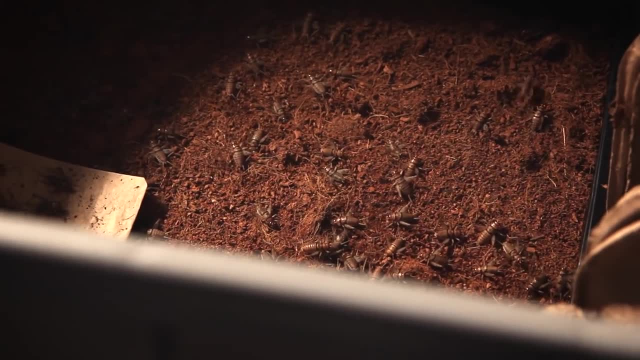 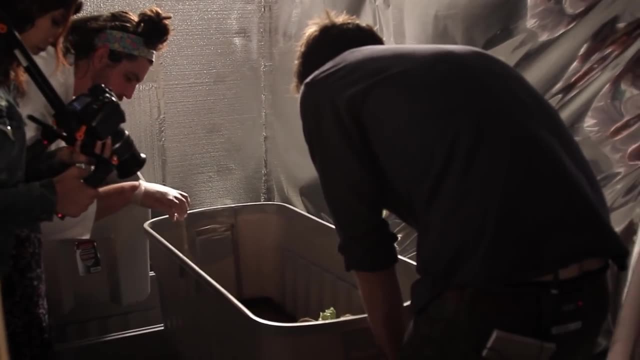 These are all mating, All these are mating. yeah, these are the brood trays, so you can see the females kind of digging around. We even see a cricket laying her eggs and it's just as spellbinding as promised. Yeah, you see the humping right.